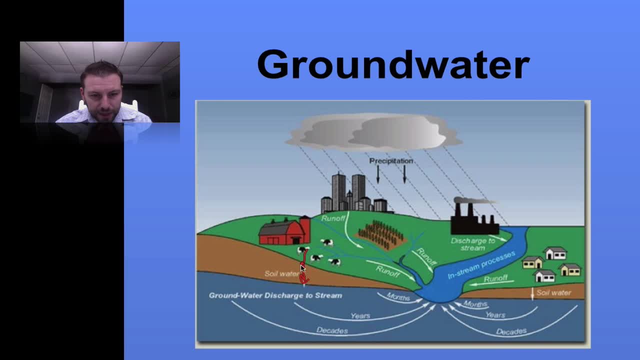 we have infiltration. Notice that as the infiltrates and percolates through the water, it fills up our zone of saturation or underneath our water table and that the water moves or the groundwater flow is basically towards these streams And that's what supplying here. This would be very similar to our upper glacial on Long Island, Not really much different. 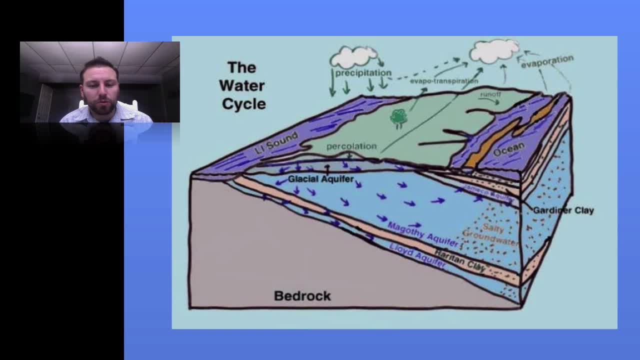 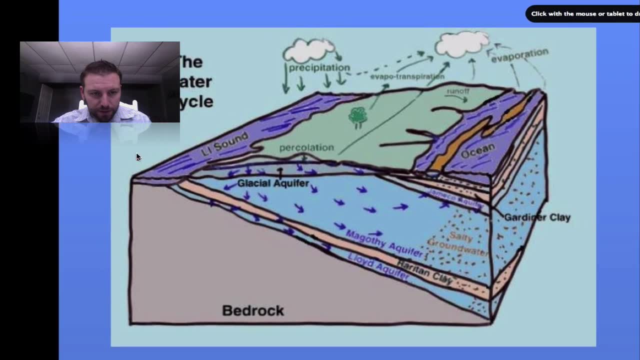 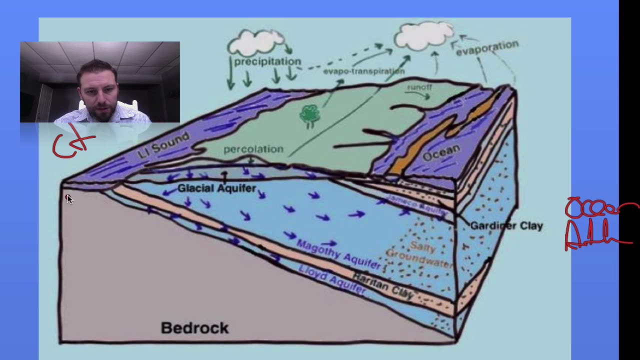 This is what the actual ground, the aquifers, look like underneath Long Island. See, here we have bedrock which slopes away, so this is like Connecticut over here, and we go out towards the ocean, the Atlantic, and notice that the bedrock tilts down. We have the. 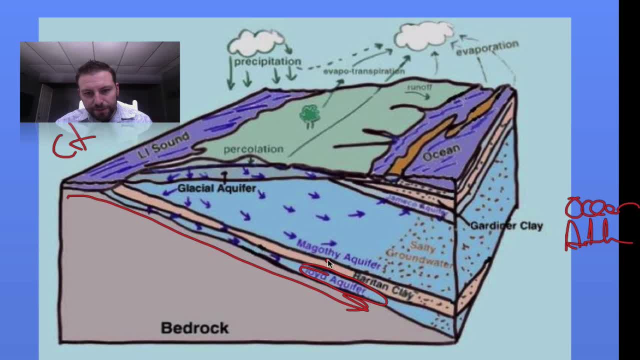 Lloyd aquifer right here, which is confined by rariton clay Clay, because of the extremely small sediment size and the pore spaces, really doesn't allow for the movement of groundwater across it. Then we have our Magothy aquifer right here. Notice it's a relatively large aquifer Once. 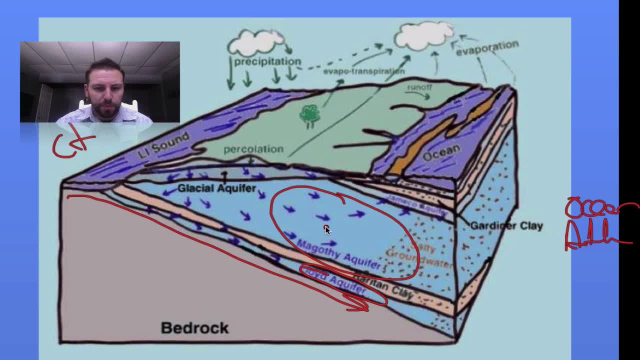 again all sediments in here that have water between the spores, pore spaces. Then our upper glacial aquifer right here- and this is the one I said- that supplies mostly our streams and rivers. There's two others, There's the Jamico right here, but for the most part we don't really. 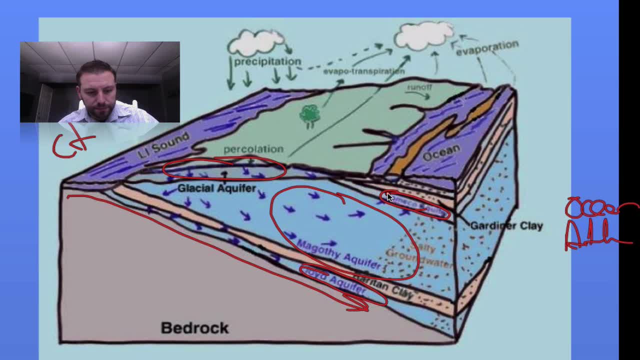 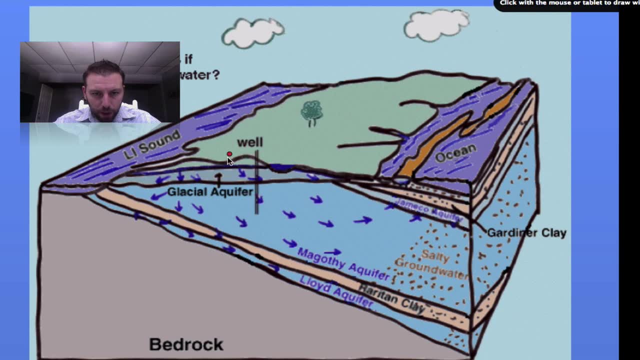 have access to this as it's underneath our barrier islands, If we pump groundwater from Long Island. So here we have a well, The water is going to come out through the well and you notice that we have a little bit of disruption of the groundwater flow. We continue to pump it'll. 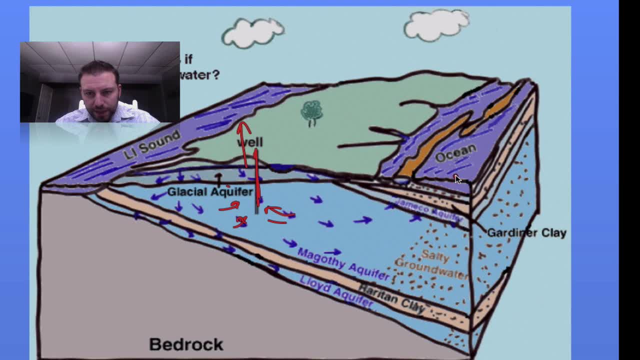 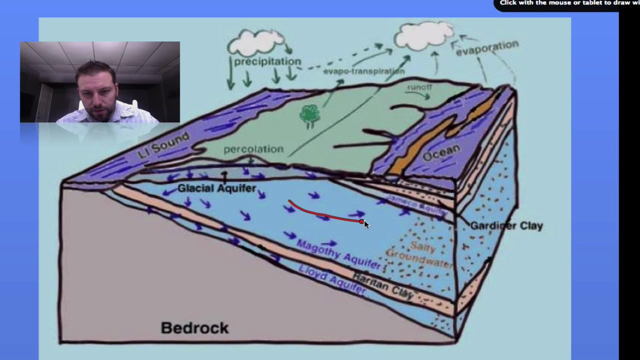 actually move inwards like this, Where we could potentially pull salt water. So for Long Island, especially communities near the, maybe towards the south shore, If there is too much pumping of groundwater it'll actually pull in salt water, But we don't have a well such as in the slide before We can actually 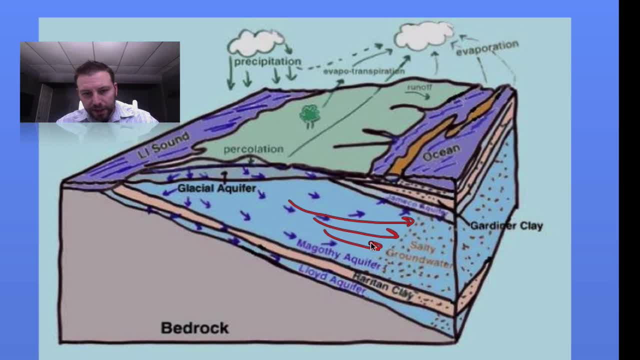 the fresh water make its way or push out any of that salt water. So there's a balance that we have to play. We want to make sure that that water that infiltrates and percolates into the ground is always there to keep salt water out. At the same token, we need to be able to use some of that water. So you have to make. 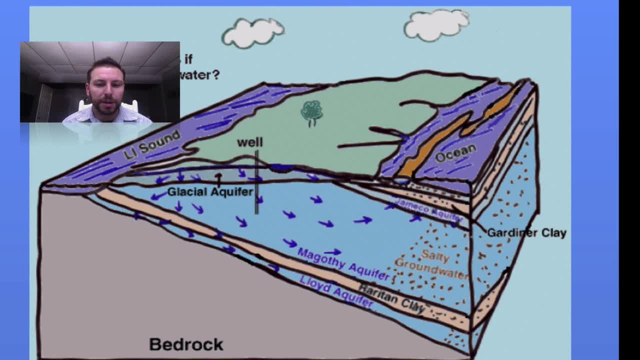 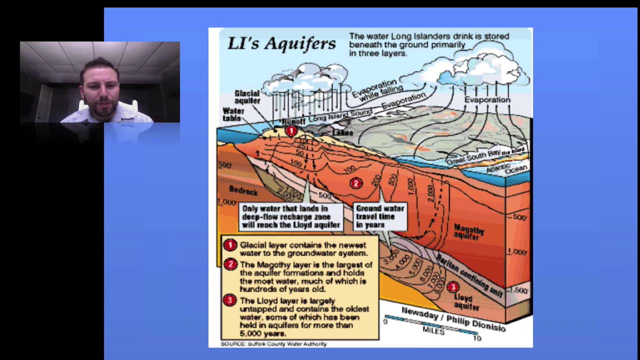 sure that we're not pumping too much to allow for the salt water to come into Long Island's aquifers. This is just taking another look at Long Island aquifers and basically the travel time or the years it takes for groundwater to move. So if you look up here, water basically makes its way. 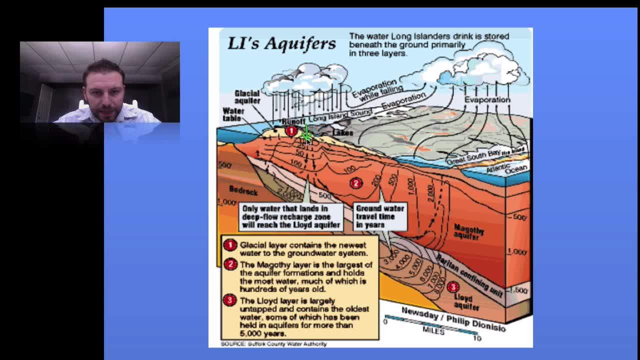 through the upper glacial in a number of years, One to ten years. the deeper we get down into, the magnify the water takes 25 years to percolate down and as it moves through, you can see, it takes longer, longer and longer. The Lloyd. 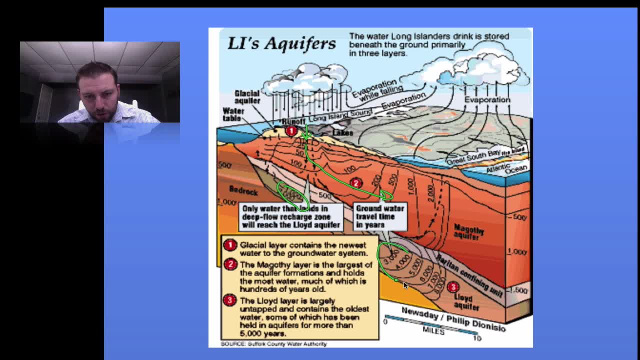 aquifer thousands of years. this water is in there for a long time, So the Lloyd aquifer are one of our oldest aquifers. Basically, the water has been there longer than most people have been around, as far as we know. There are a couple of different ways we use water. We alluded to basically that we 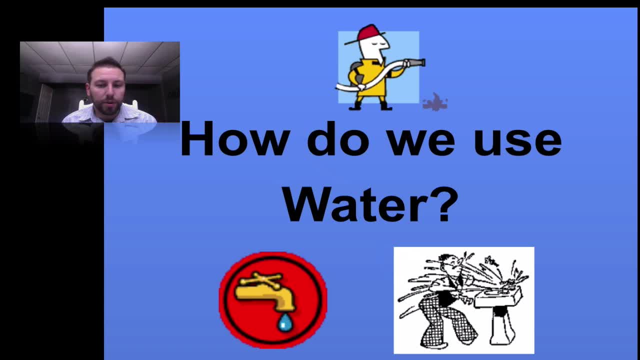 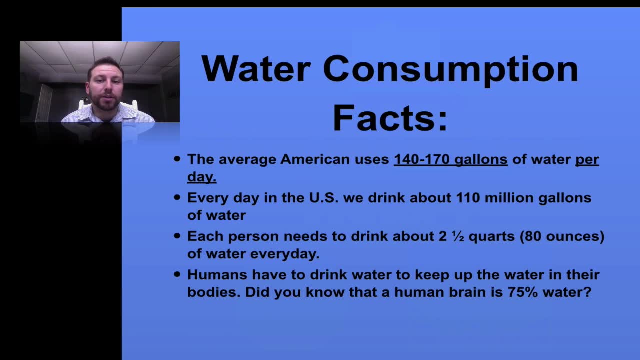 can pump from the hose outside or from water inside the house. Here are just some water consumption facts. Basically, average American uses about 140 gallons of water per day. It's quite a bit. in the US we drink about 110 million gallons of water. But that stuff you know, we, I 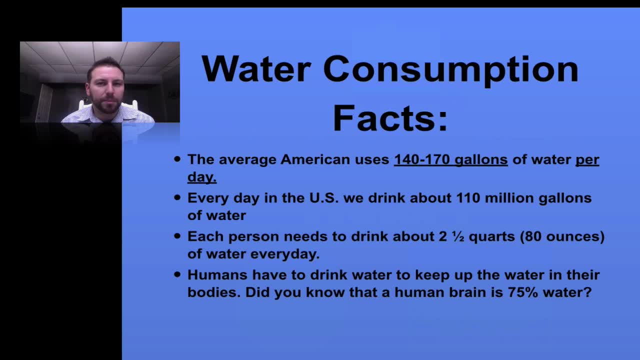 think most people know about how much water we need- about 80 ounces per day. But the biggest fact this this hundred and forty gallons of water per day because we can change the amount of water that we're using. if you take a look at this, you can see some. 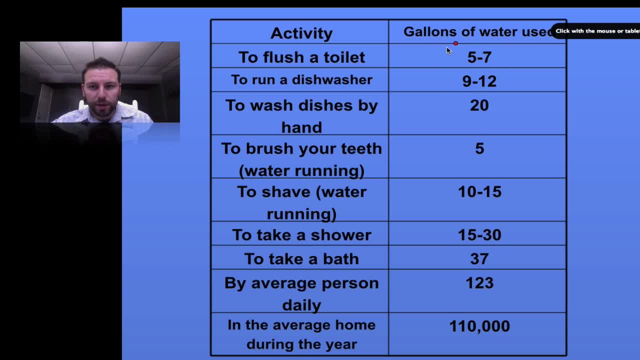 averages it takes from gallons of water use flush toilet about five gallons, shower 15 to 30 or a bath 40 gallons. so these areas are where we could try to cut back and save a little bit water. for instance, if we just get rid of a bath, we 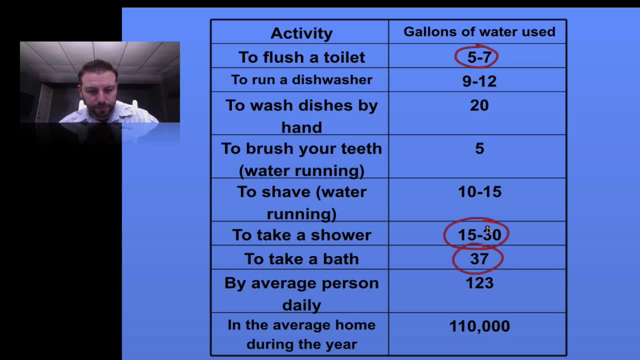 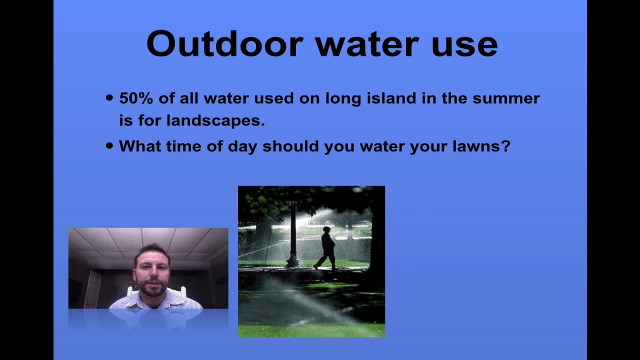 can save the amount of water we're using and take shorter showers outdoor water use. here on Long Island, we are watering our lawns quite a bit, so that's what you're gonna see during the summertime: a lot of use of waters, and in Garden City, as we know, you can only water your lawn on alternate days. that. 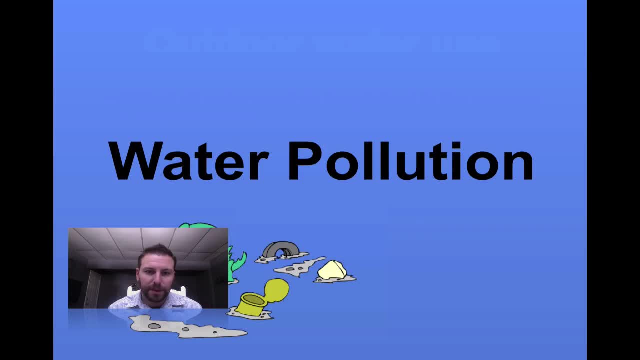 is to cut down on the amount of water that people use. that's about it. we're gonna hold off on water pollution until next time. I hope you enjoyed this screencast. take care.